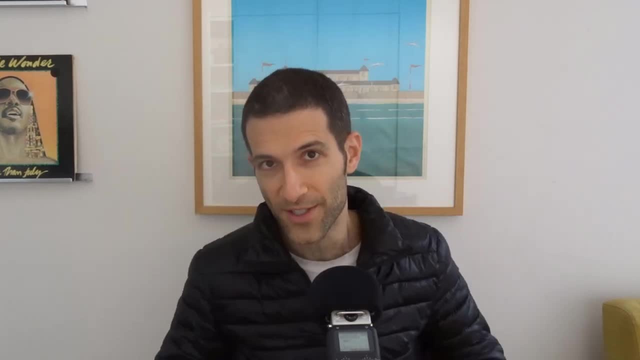 Type 1 and Type 2 errors are critically important to the study of hypothesis testing, but they're often quite misunderstood, as is the concept of statistical power. So this particular video is dealing with all three of those in a really neat way. 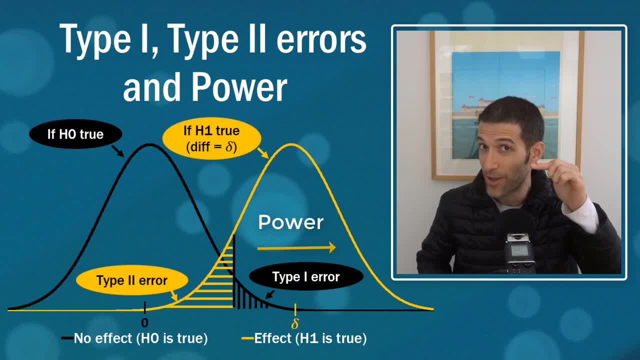 and hopefully by the end you're going to be understanding exactly what this graph is all about, this one over here. If it doesn't make any sense to you just yet, don't worry, I'm going to lead you through it. And in fact it's only when I myself started teaching. 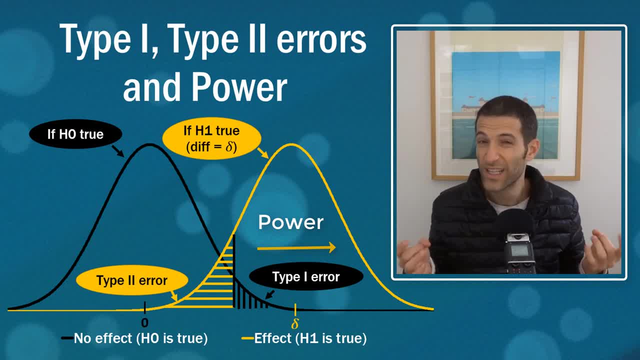 this exact topic, that I understood some of these concepts really for the first time, So hopefully I'll be able to open the window a little bit for you so that you can grasp things fully. My name is Justin Zeltser. it's zstatisticscom. 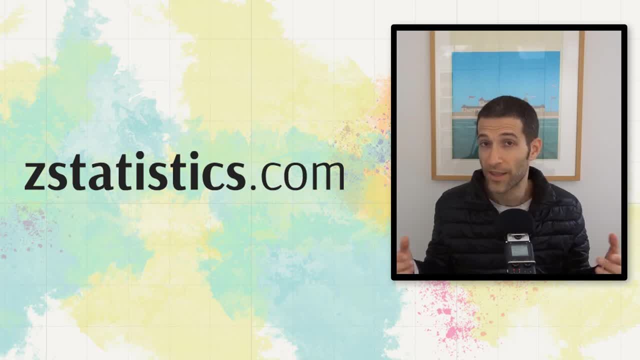 If you like this stuff that I do, feel free to tell a friend so the audience can grow and I can keep making videos like this. or you can just like and subscribe, do all those kinds of things, But But otherwise come with me and let's explore Type 1 and Type 2 errors. 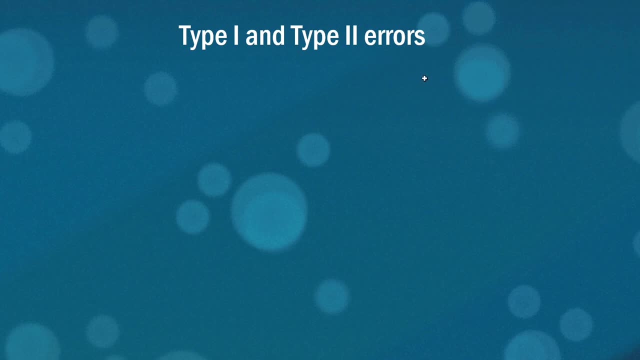 Okay, so Type 1 and Type 2 errors are firmly entrenched within the concept of hypothesis testing. So we need to do a bit of a recap on hypothesis tests, And I think the best way of doing that is using the classic court case example, where 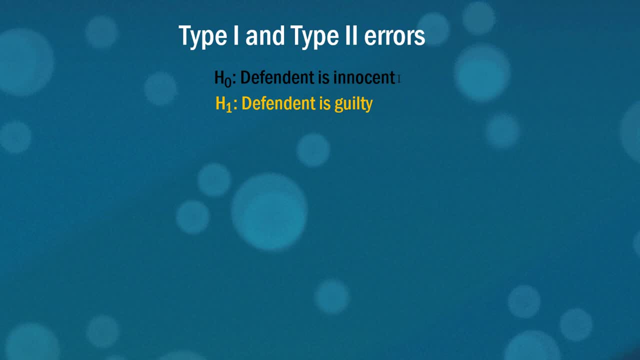 there's a defendant on trial and we're going to give them the benefit of the doubt, So they're going to be innocent until proven guilty. So what we do is we in our null hypothesis- this top line is called a null hypothesis. 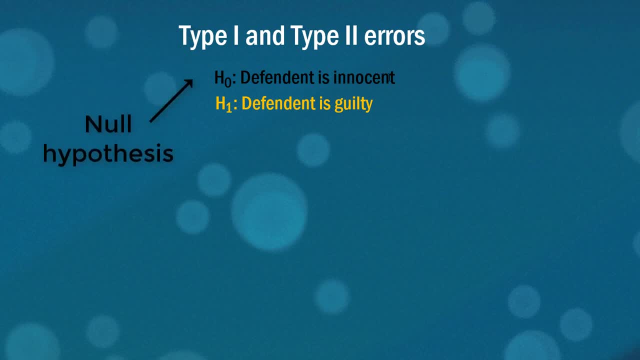 we say that the defendant is innocent And we want to see if there's enough evidence to move from the null hypothesis to our alternate hypothesis state And realistically, it is this alternate hypothesis that we are seeking evidence for. So it's important to note that the default setting or null hypothesis is the reverse. 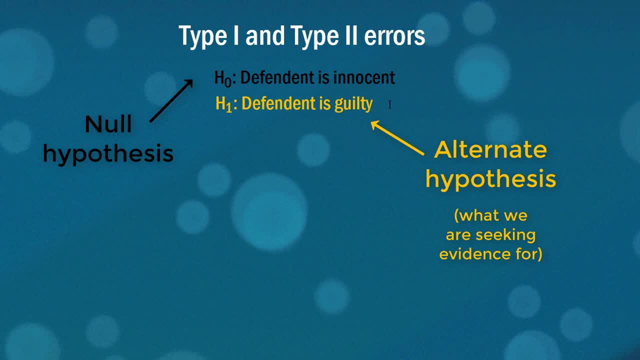 of what we're seeking evidence for. We always are. So we start with the assumption that the person is innocent in this case and we're going to see if there's enough information to show that they're guilty. And this process of being conservative is common to both the courtroom and also to doing 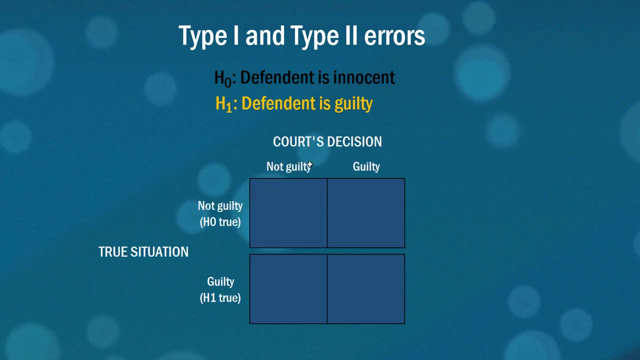 statistical hypothesis tests. So these four boxes represent the possible outcomes from a criminal trial. Let's consider the case where the person is actually not guilty. Now, we can never know whether the person is not guilty or not, But let's just say that this person happens to be not guilty. 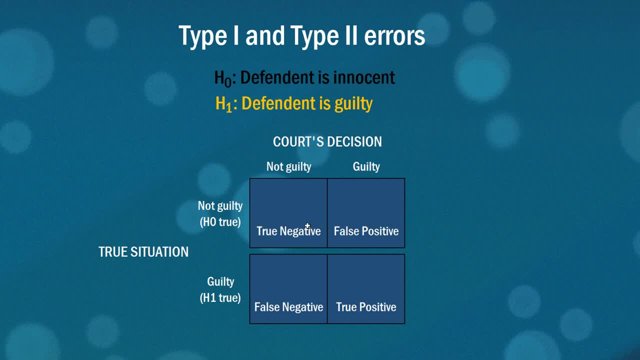 If the jury pronounces them not guilty, then we've made what's called a true negative. We've correctly identified a lack of guilt or a negative right. So we haven't been able to budge from this null hypothesis. And it was correct for us not to budge from that null hypothesis. 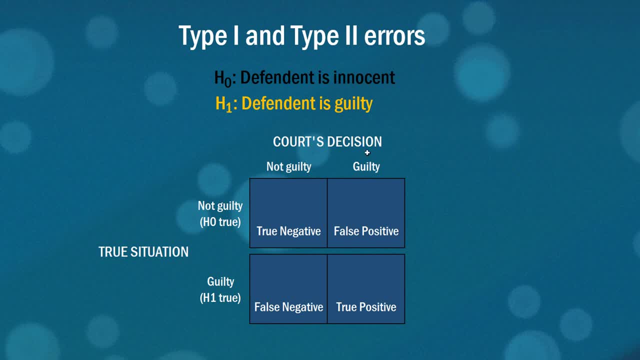 Now, a false positive means that we've actually falsely decided that this person is guilty, when in fact they happen to be not guilty. That's called a false positive. And for the same reasons down here, when the person happens to be guilty and we've called 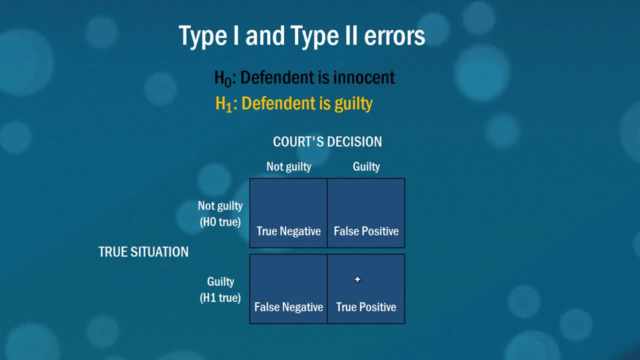 them not guilty. that's a false negative. And then, of course, we have a true positive, down in this bottom right corner, where we've correctly rejected that null hypothesis, to say that, yes, this defendant is guilty. Now it's important to realize that in these two cells, the ones on this off diagonal, 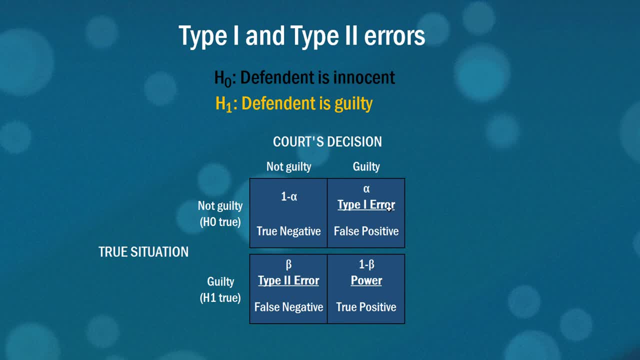 we're actually committing an error. In the top right There's a type one error And that means we've incorrectly rejected this null hypothesis And that's given the Greek letter alpha. It's also actually called the level of significance And, as we'll see, in a test for significance we can actually set that to be whatever we 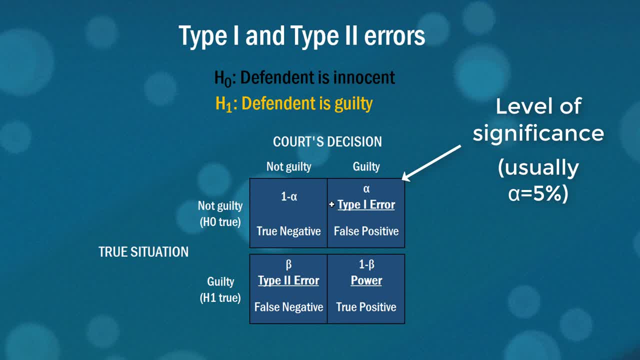 like It just depends on how strict we're being with the evidence we require to reject that null hypothesis and pronounce this person guilty. Now a type two error is also, given the letter beta And that's when the person was guilty, but we just didn't have enough evidence to find. 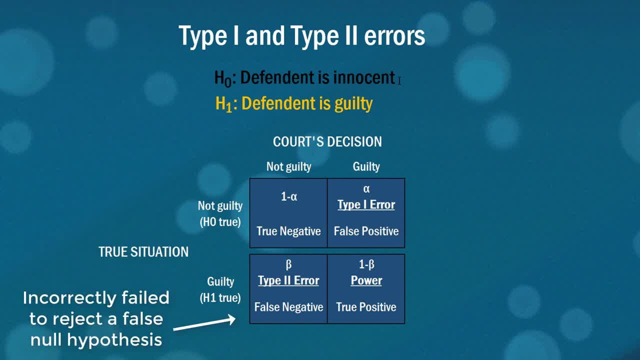 them guilty, So we've incorrectly failed to reject the null hypothesis. Now we also get this thing called power, which is the ability of the test to correctly reject a false null hypothesis If the person was guilty. the power tells us how likely we are to correctly convict. 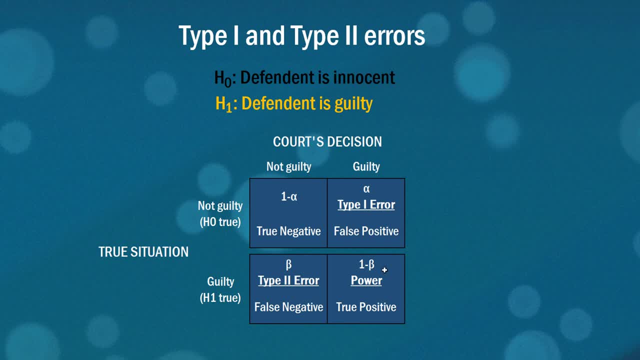 them. Now be aware that beta plus one plus beta is equal to one. Similarly, beta plus one plus beta is equal to one. One minus alpha plus alpha is equal to one. So these are the probabilities looking across these rows, But let's put this into a more general hypothesis test that is used across the statistical spectrum. 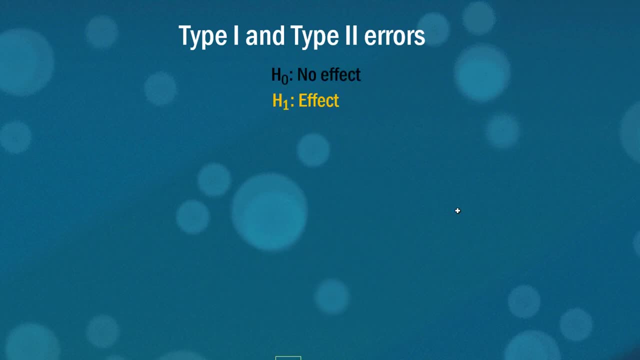 And I've generalized this hypothesis test such that the null hypothesis is simply that whatever we're testing has no effect, And the alternate hypothesis is simply that there is an effect. Now there are numerous hypothesis tests that fit this description. For example, in the medical world, you might be testing for an intervention and the null 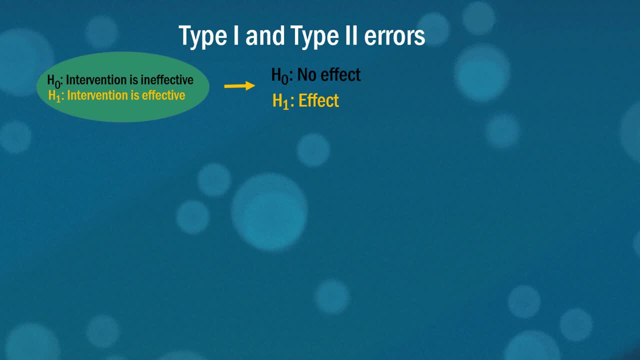 hypothesis might be that the intervention is ineffective, or in other words has no effect, And the alternate is that the intervention is effective. Other examples are diagnostic tests. So say, we're looking at testing for COVID, right, The person either has COVID or they don't, and the diagnostic test could either come. 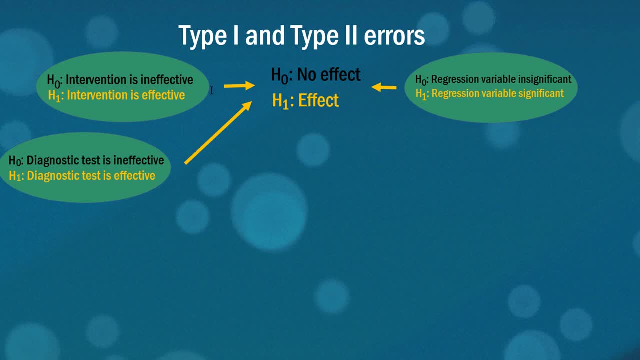 back positive or negative. Other examples are in regression. If we're looking at particular variables, We might, in the null hypothesis, consider them insignificant and we're going to see if there's enough evidence to suggest that they are significant. And a final example are when we are comparing group means. 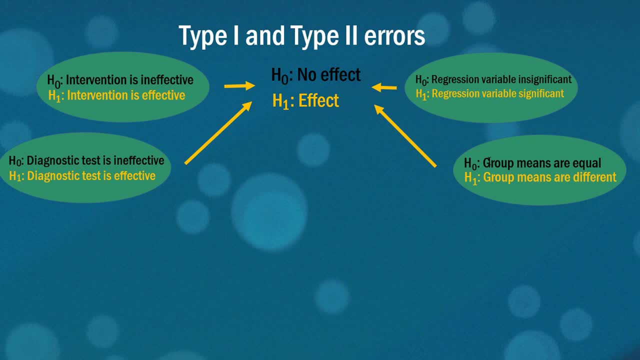 So two different groups or two different treatments are being compared and we want to see whether their means are equal And the alternate hypothesis will be that the means are different And you can see that in each of these cases the null hypothesis is almost like our conservative. 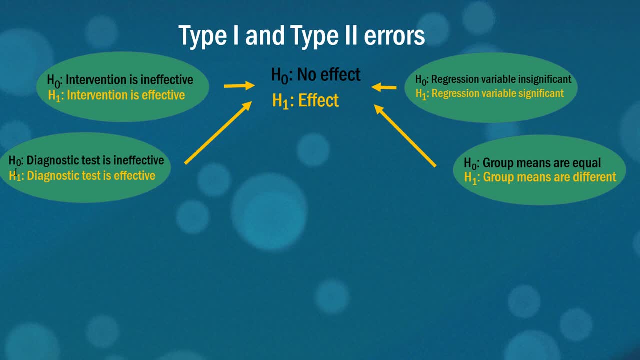 starting point. We really want to show that there is no effect. We want to show that the alternate hypothesis is true. but because we're statisticians, we're always conservative and we make our default hypothesis or our null hypothesis to be that there is no effect. 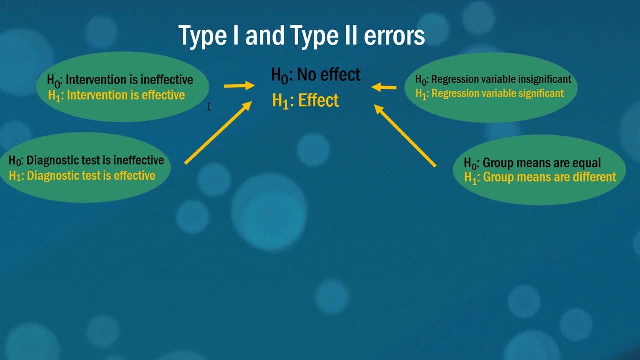 So pretty much every hypothesis test is going to fit this description, And what we'll have is a again a true situation in which we can never know. And then we have our sample results. So we usually take a sample of something and try to assess, using that sample, whether there 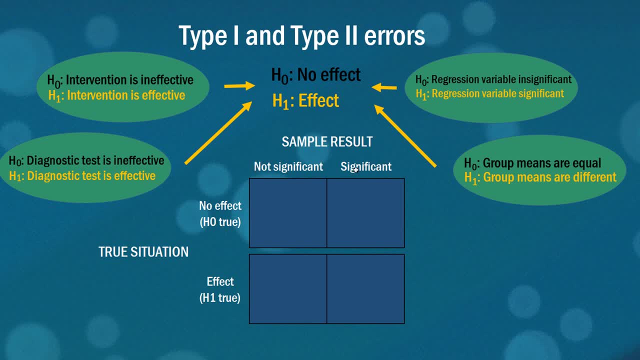 is an effect or not. or we can say that the effect is significant or not significant. So I'm hoping you're seeing the similarities between this and the courtroom example. but you can see we've got the same things. We've got our false positives and false negatives called type one and type two errors. 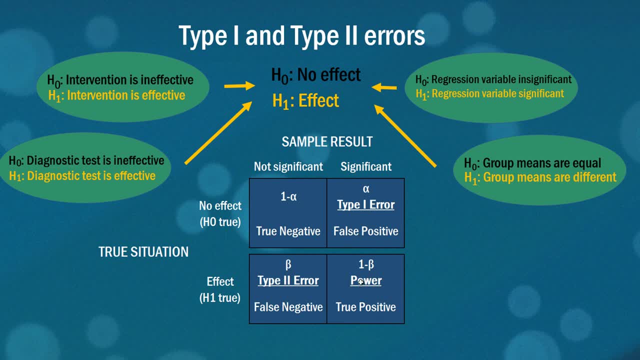 And again, we have this power down here as well, which, again, is the ability of the test to find an effect, if indeed there is one. Okay, So let's see how this actually plays out. Okay, So let's get our hands out with an example. 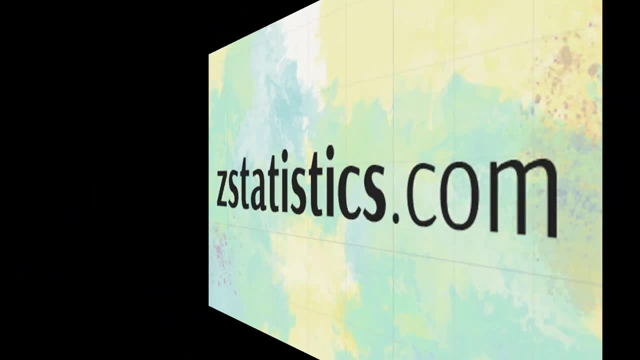 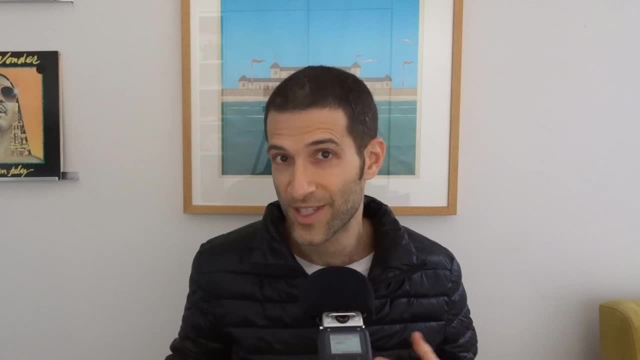 Now, before we get to the practical example, I thought I'd do, for the first time, a bit of self-promotion. I've got a website called ZedStatisticscom which has a whole heap of categorized statistical videos. You can see them here. 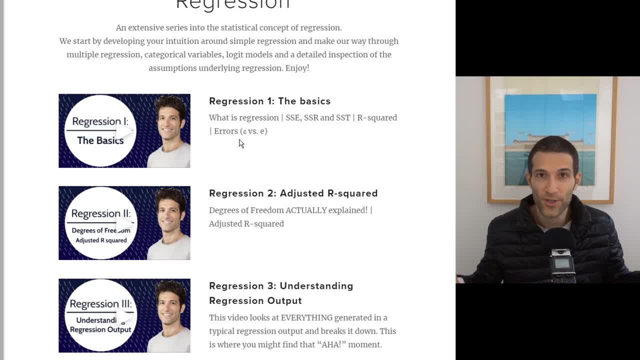 I just thought I'd let you know, in case people are like: what is this guy? What's he doing? Just putting up videos all the time. I'm in the process of putting together what I hope to be a nice, complete, practical example. 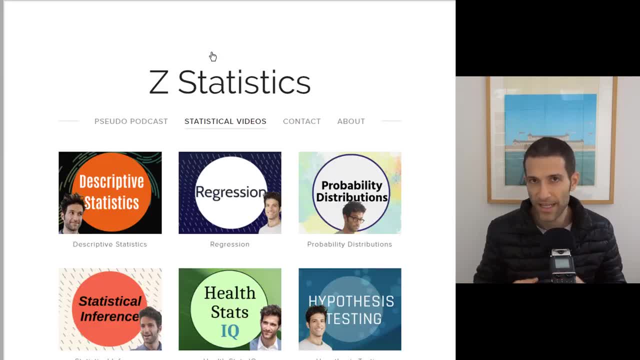 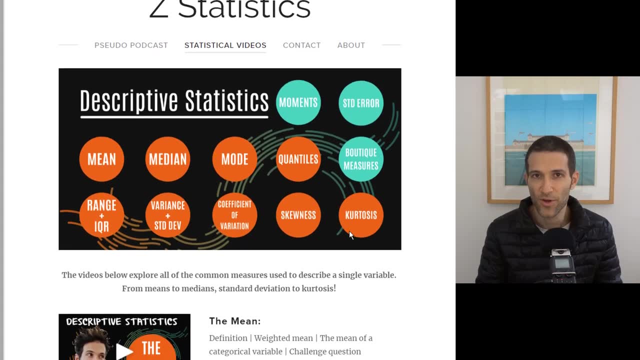 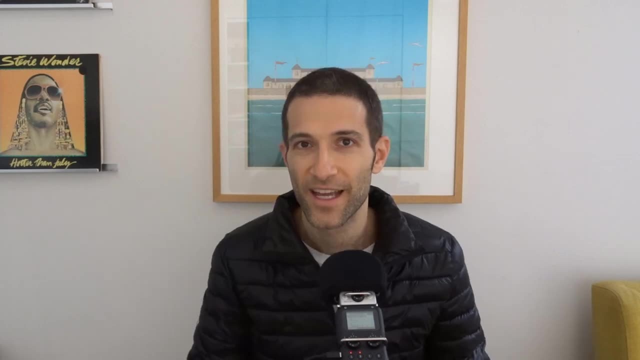 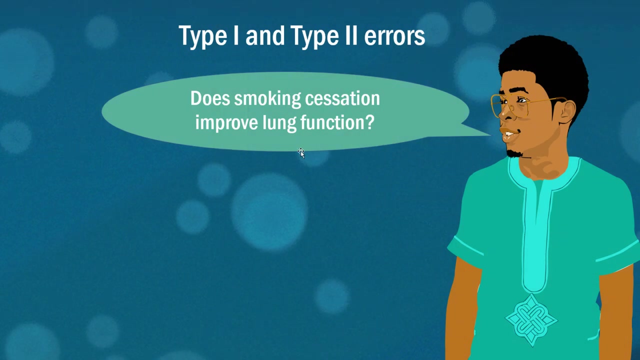 Okay. So let's get back to the video and take a look at the example that we're going to be using, which is all about smoking cessation and whether that improves lung function. Let's check it out, Okay. So if we're talking about smoking cessation, or in other words, whether stopping smoking, 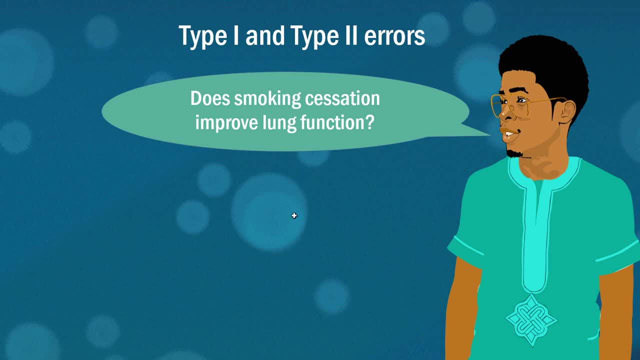 improves your lung function. we need to set up our null and alternate hypotheses, And because we're conservative, we're going to go with the null hypothesis being that there is no effect of smoking cessation on lung function. And here I've just said that the difference is zero. 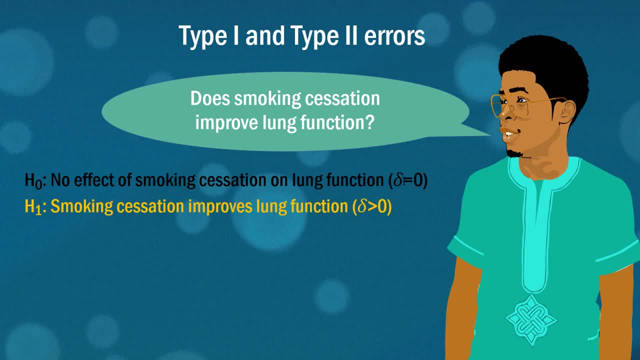 That's what that curly Greek delta represents: The difference in lung function between those that stop smoking and those that continue smoking. And our alternate hypothesis, which is the thing we are seeking evidence for, is that it improves lung function. So again, it's that common conservativism where we put the no effect in the null hypothesis. 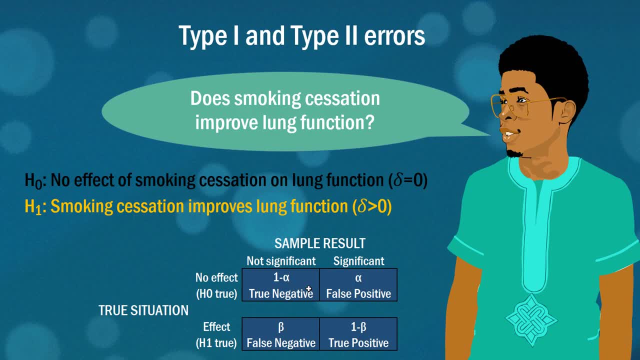 to see whether we have enough evidence to reject it, And then we can set up our two by two table again, if we like, with the true situation over here, which is the reality of the effect of smoking cessation on lung function and then our test result, what we actually find from this test we're about to do. 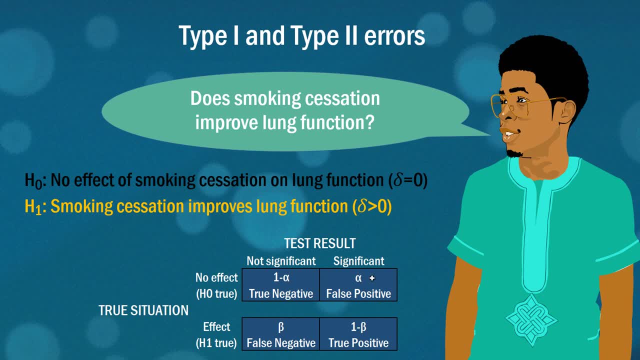 Now that's all well and good, but let's go a little bit deeper and see how we can derive how big some of these probabilities are, such as the probability of a type one and type two error, and also have a look at the power. 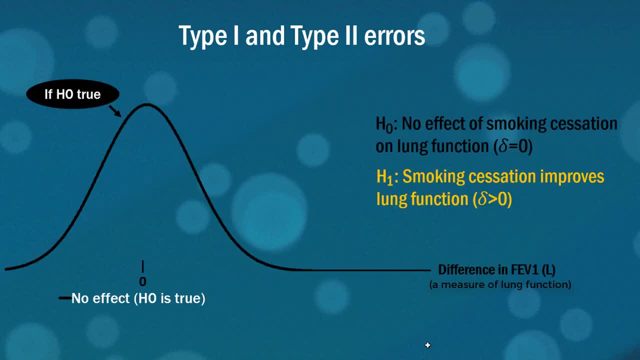 So this is where it's going to get good people. Okay, so this is my favorite bit- We've got our null hypothesis that there's no effect of smoking cessation on lung function. In other words, the difference this is delta. 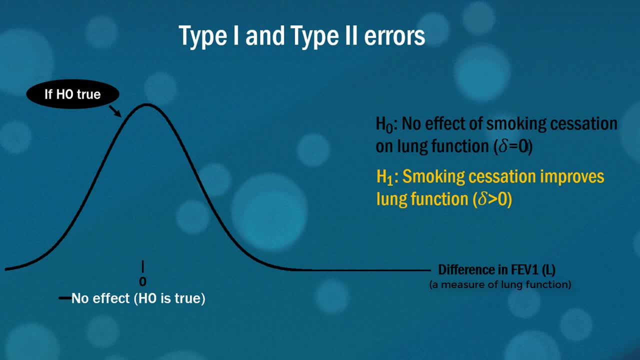 The difference is actually equal to zero. Now let's think about this for a minute. If the true difference was exactly zero, meaning that whether you smoke or you stop smoking, it doesn't affect your lung function- Imagine you took a sample. Would you expect the sample difference to be zero? 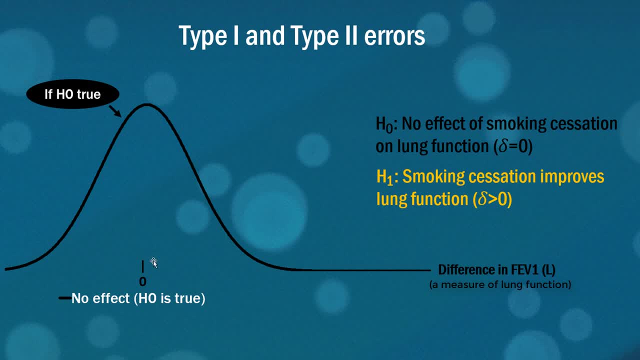 You probably expect some kind of random variation in your sample, right, It wouldn't be exactly zero. Potentially, those that stopped smoking in your sample might have a slightly higher lung function, Or maybe they might even have a slightly lower lung function than those that kept smoking. 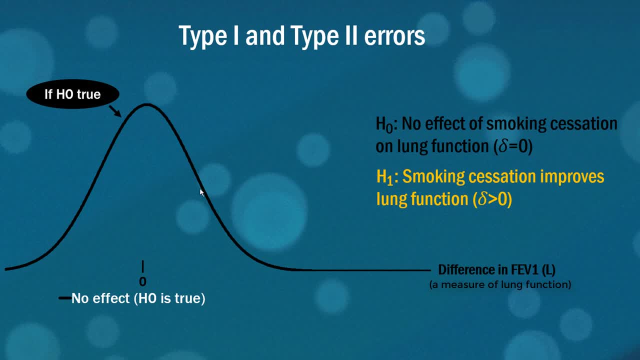 Because when we take a sample we are susceptible to all the random variation that sampling entails. They very rarely match up perfectly with the mean of the population. So what a hypothesis test is going to do is set up this region up here, which usually 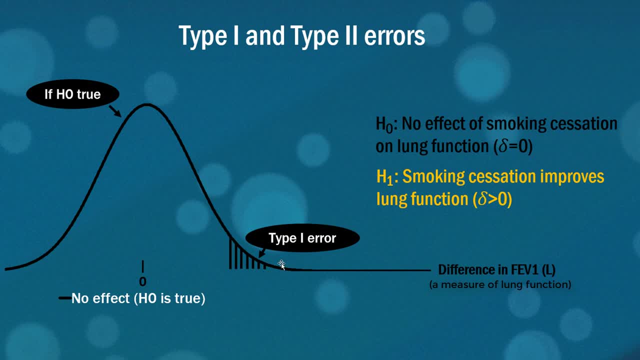 is given a probability of 5%, So that would be 5% of the total area of this curve. Okay, So we're going to set for ourselves the probability of incurring a type 1 error, And that basically means that if our sample mean is too extreme- say it's up in this black- 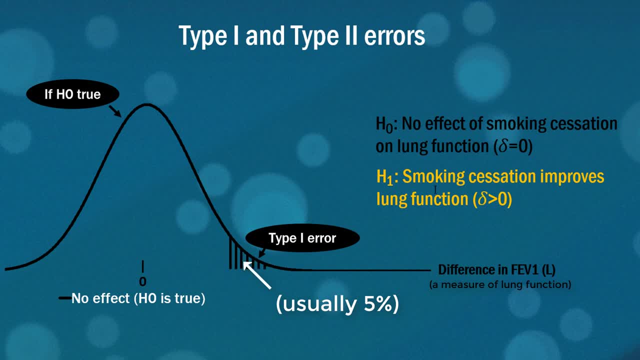 shaded region. we're going to reject the null hypothesis. But don't forget, it's entirely possible that we're rejecting a true null hypothesis And this black curve is indeed that situation where the null hypothesis is true. So it's almost like we allow ourselves a 5% chance of success. So we're going to set for ourselves the probability of incurring a type 1 error, And that basically means that if our sample mean is too extreme- say it's up in this black shaded region- we're going to reject the null hypothesis. 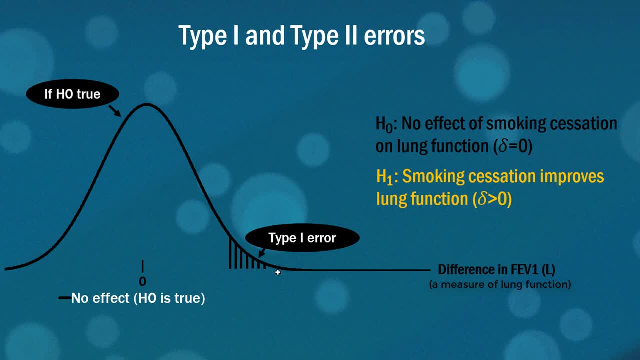 But don't forget, it's entirely possible that we're rejecting a true null hypothesis And that basically means that if our sample mean is too extreme- say it's up in this black shaded region- we're going to reject the null hypothesis And that basically means that if our sample mean is too extreme- say it's up in this black. 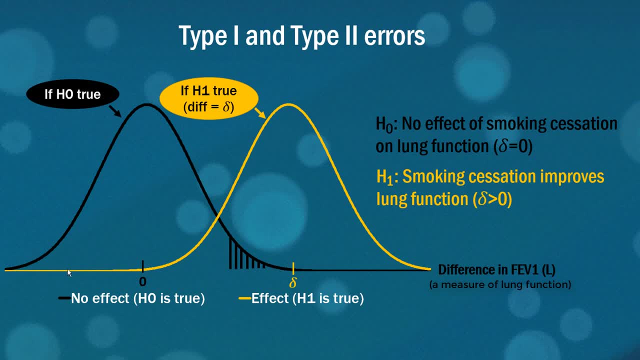 shaded region. we're going to reject the null hypothesis, So we're going to set for ourselves the probability of incurring a 5% chance of getting it wrong, But that's something we just have to live with right Now. here's the best bit. 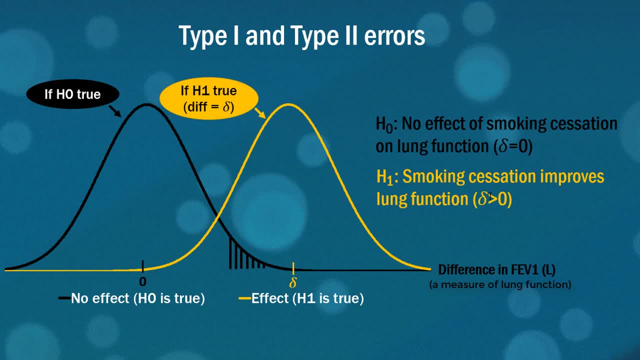 Let's now presume that, in fact, the alternate hypothesis is true. So if it was true, then there's going to be some difference in the lung capacity or lung function of those people that stop smoking versus those people that keep on smoking. So if indeed there is an increase in lung function, this yellow curve must exist somewhere. 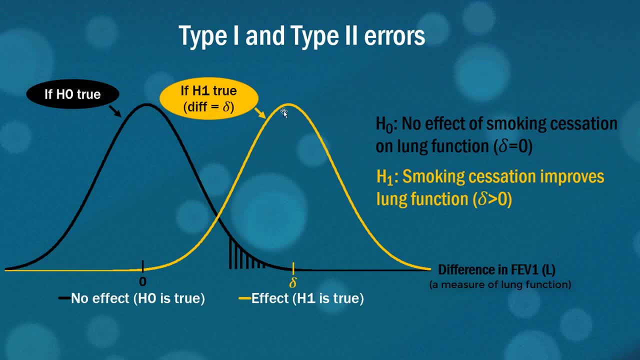 right. This must be the true representation of the possible outcomes from our sample. Our sample is not centered at zero. our sample, in reality, is centered at delta. So what happens then is that if you look to the left of this black line- don't forget, 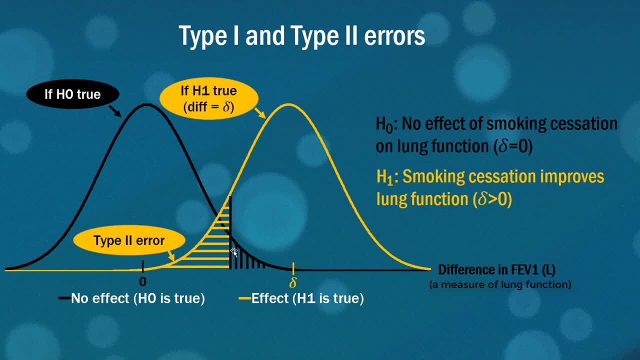 this is where we had our type one error. the black bit here was our type one error. That's where we would reject the null hypothesis. To the left of that point we are not rejecting the null hypothesis right. So if we do not reject the null hypothesis for the purpose of this yellow curve, that's. 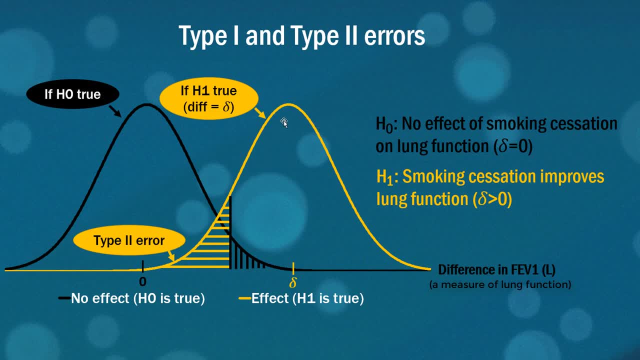 us committing an error because we now know, given this yellow curve, that there was a difference. So if we've failed to reject it, this is the area which is going to result in us committing what's called a type two error. So if we put the type one error label back, you can see it's quite neat. 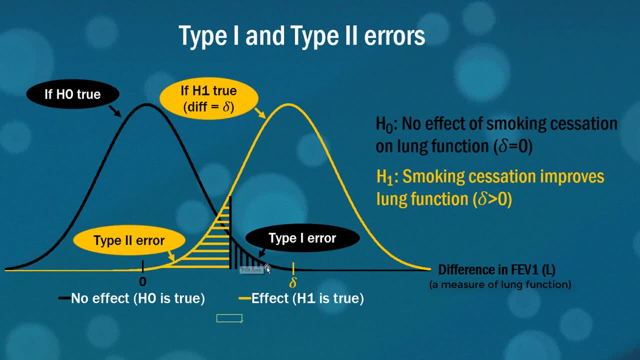 We've got this type one error, which we've defined from the level of significance of our hypothesis test, And wherever that line goes, that starts, this rejection region to the left of that will be where we have a type two error in terms of this yellow curve. 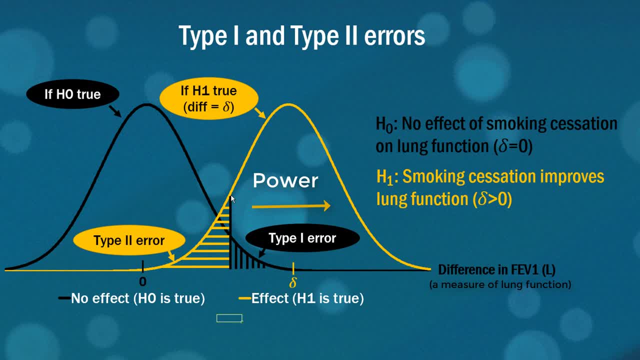 So where's the power in all of this? Well, the power is everything else in this yellow curve, So it's this whole region. here is our power: essentially one, minus The area in the type two area. Now, I actually found this really great as an explanation for how all these things interrelate. 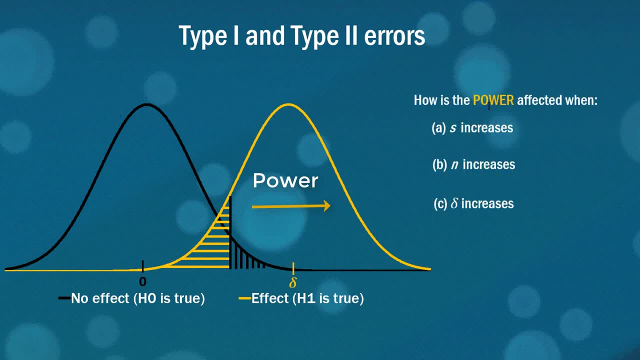 And so it's probably worthwhile you thinking about this now. I've got three questions for you And hopefully you can pause the video when I ask them and have a real think about them before I reveal the answer. But I want you to think about how the power which is, in fact, this region here, how is 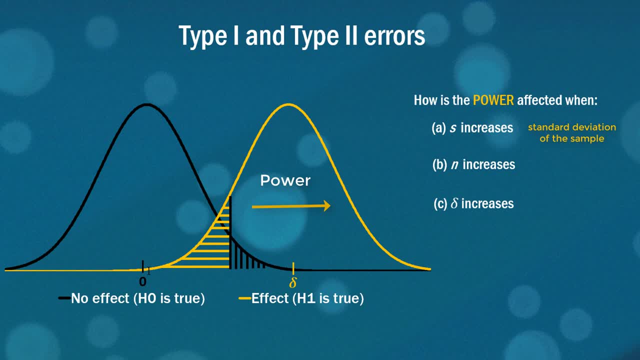 the power affected when S increases. S is the underlying standard deviation, S is the deviation of our sample. Now, with more variation and uncertainty in our sample, these curves are going to become fatter. And if we hold everything else the same, you can see that the area of overlap is going. 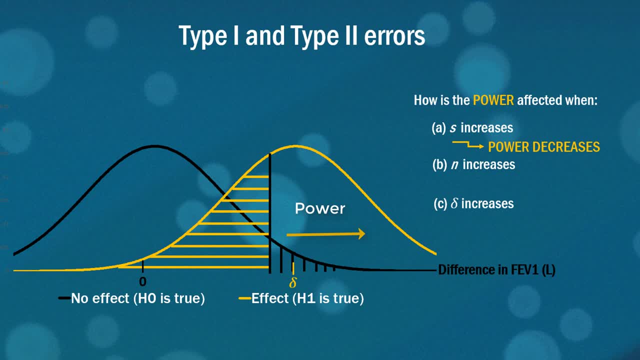 to increase. Therefore, the power will have to decrease, As you can see that the power now takes up a smaller proportion of that yellow curve. Now what happens when N increases, which is your number of observations in the sample? Again, pause the video and have a think about how that might play out.